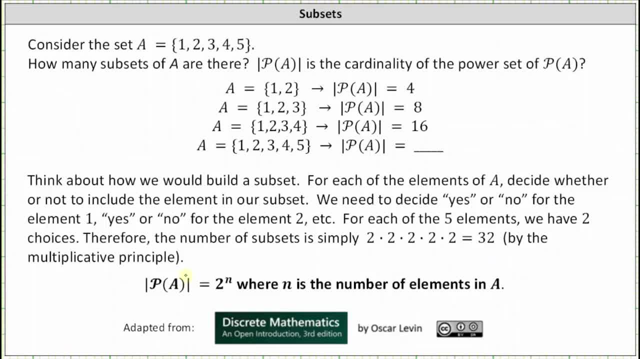 or counting principle. So we can generalize and say the cardinality of the power set of A is equal to two, to the power of N, where N is the number of elements in set A And now of the 32 subsets of set A. 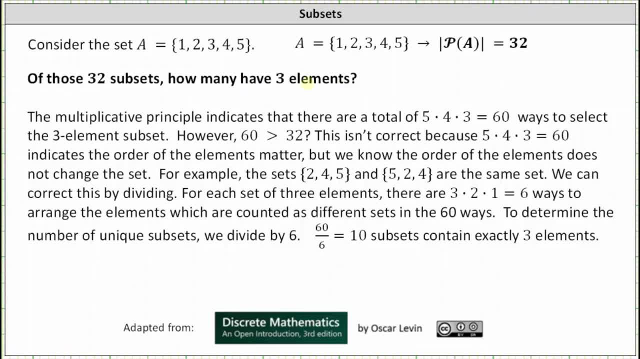 how many have three elements? We might be thinking that the multiplicative principle indicates that there are a total of five times four times three or 60 ways to select three element subsets. but this isn't quite right because notice 60 is greater than 32,. 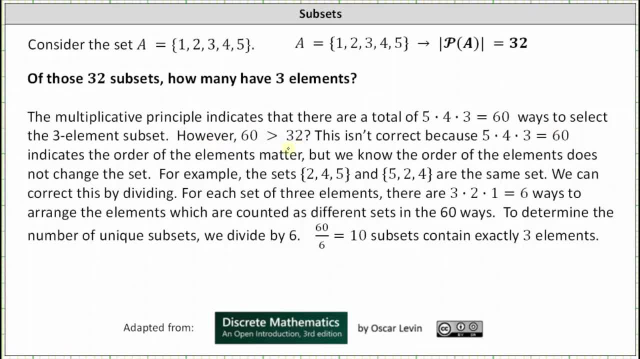 and we know we have a total of 32 subsets. This isn't correct because five times four times three equals 60, indicates that the order of the elements matter. but we know the order of the elements does not change the set. For example, notice these two sets: 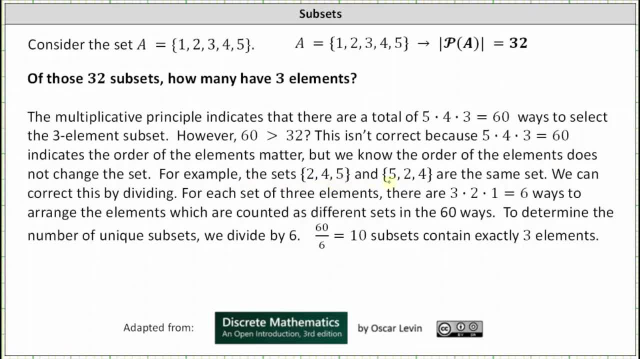 with the elements of two, four and five are the same set, but in the calculation of five times four times three, which gives us 60, these would be counted as different. However, we can correct this by dividing For each set of three elements. 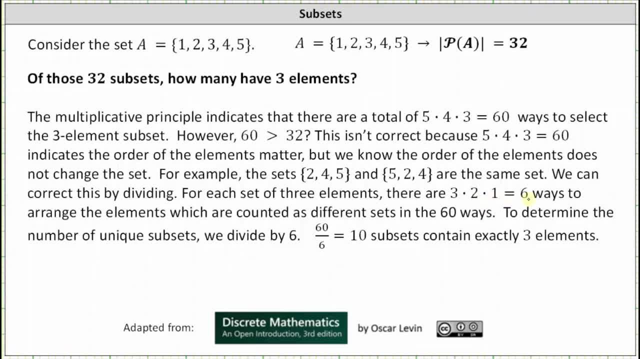 there are three times, two times one or six ways to arrange the three elements which are counted as different in the 60 ways, And therefore we can determine the number of unique subsets by taking 60 and dividing by six, which gives us 10 subsets. 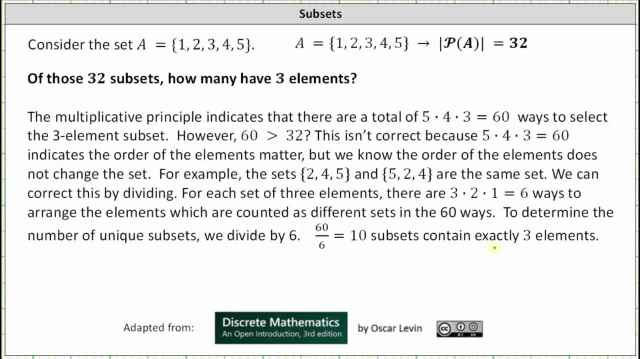 which gives us 10 subsets with exactly three elements. Before we look at an easier way to determine the number of subsets with a certain number of elements or a certain cardinality, let's look at a table. Let's complete the table below: where, in the first row, 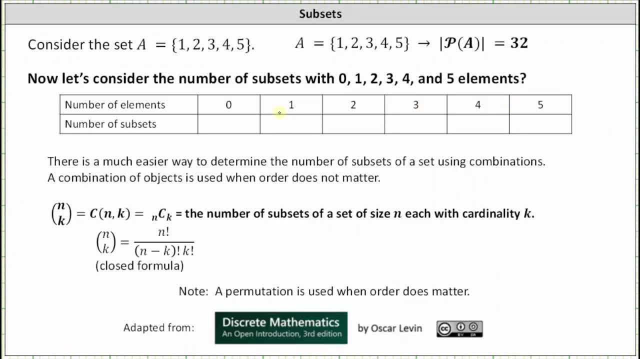 we have the number of elements in the subset and then the second row, we have the number of subsets. For example, how many subsets of set A have zero elements? That would just be one set, the empty set, And we can also easily determine the number of subsets. 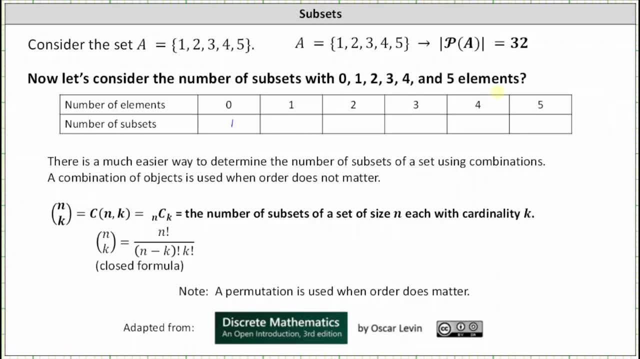 with five elements, which would be set A itself, And therefore there's only one subset with five elements. And now let's go back to the number of subsets with one element. Well, because there are five elements, there would be five subsets with one element. 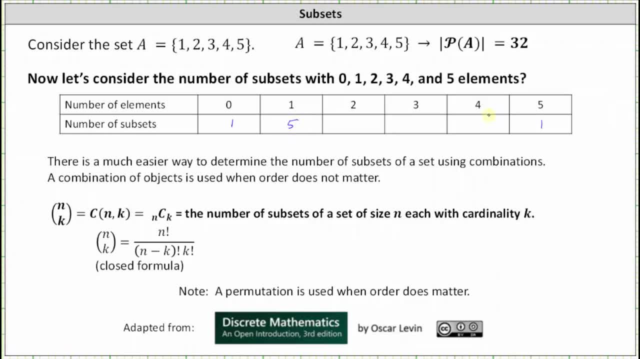 And if we think about this for a moment, the number of subsets with four elements is going to be the same as the number of subsets with one element. Every time we form a subset with one of the five elements, we leave behind four elements that would form a subset. 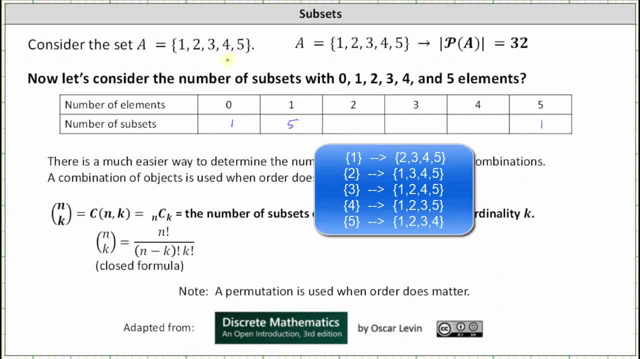 And therefore there's also five subsets with four elements And therefore there's also five subsets with four elements. This also indicates that the number of subsets with two elements and the number of subsets with three elements is going to be the same, And again, that should make sense. 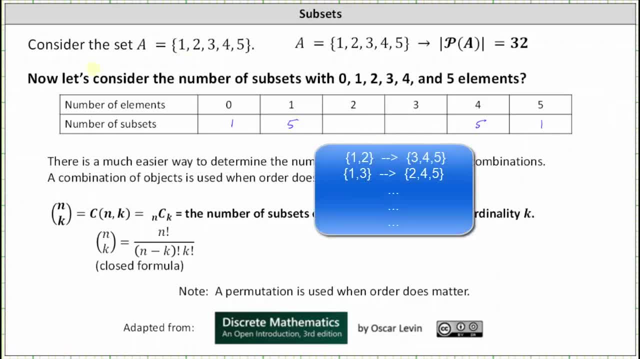 If we take two of the five elements to form a subset with two elements, the three elements left behind would form a subset with three elements. So notice, so far we've counted six plus six or 12 subsets And because we know we have a total, 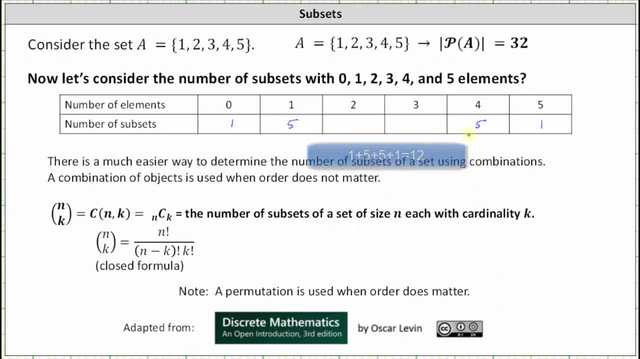 of 32 subsets. 32 minus 12 is 20, 20 divided by two is 10, which leaves us 10 subsets with two elements and 10 subsets with three elements. But there is a much easier way to determine the number of subsets with a certain number of elements. 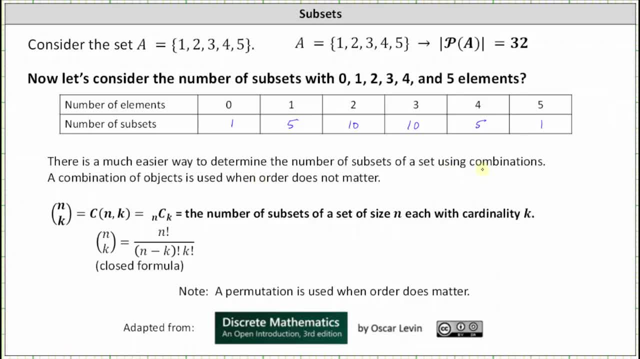 or certain cardinality using combinations. A combination of objects is used when order doesn't matter. The number of subsets of a set of size, n, each with cardinality k, is equal to n. choose k indicated by any of these three notations here. 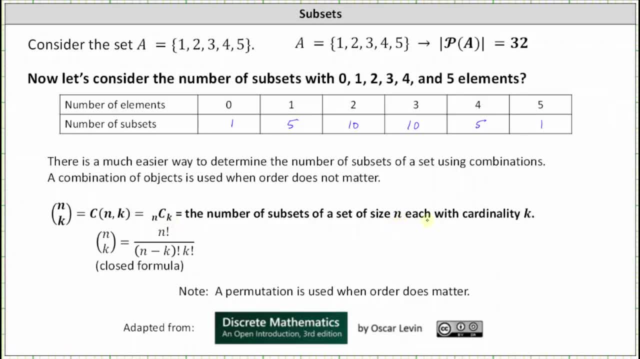 So again, n is the number of elements in the original set and k is the cardinality or size of the subset. And we define n choose k or n items chosen k to time as n factorial divided by the product of n minus k factorial. 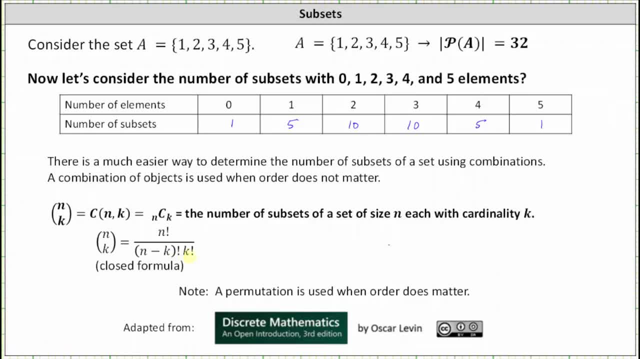 and k factorial. Let's verify the formula by verifying that for a set a, there are 10 subsets with two elements. Because set a has five elements and we're trying to determine the number of subsets with two elements, we need to calculate five, choose two. 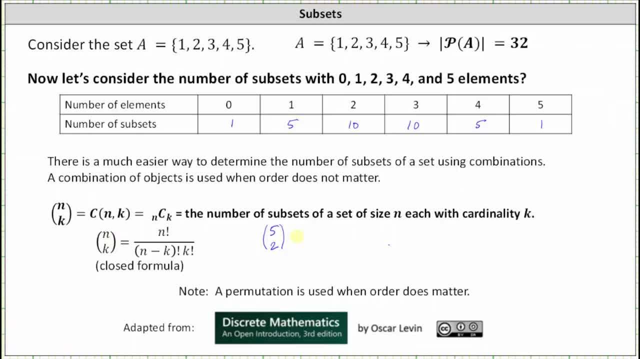 which means n is equal to five and k is equal to two. Applying the formula, we have n factorial, which is five factorial, divided by the product of n minus k factorial, and k factorial, which is five minus two factorial and two factorial. 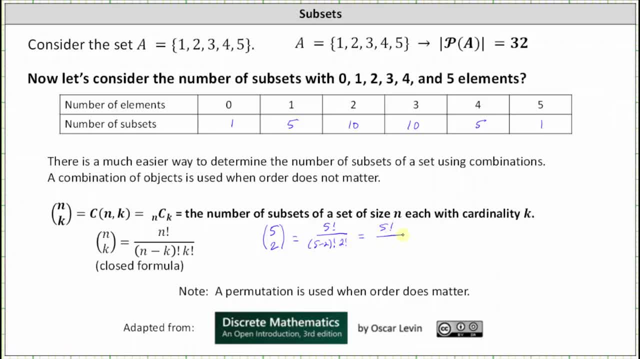 Simplifying, we have five factorial divided by the product of three factorial and two factorial. And now we'll go and expand the factorials. Five factorial is five times four times three times two times one. Three factorial is three times two times one. 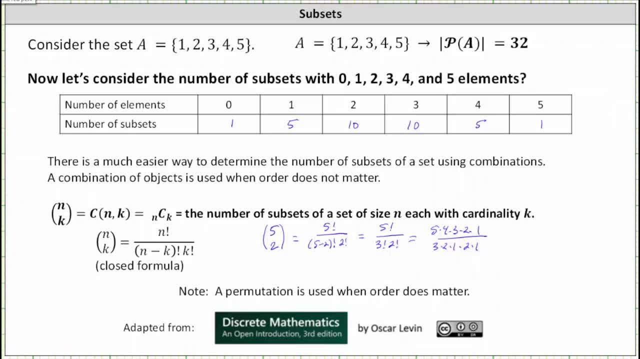 and two. factorial is two times one. And now we'll go ahead and simplify. Three divided by three simplifies to one. Notice in the denominator we have two times two, which is four. Two times two is one. Two simplifies to one in the denominator. 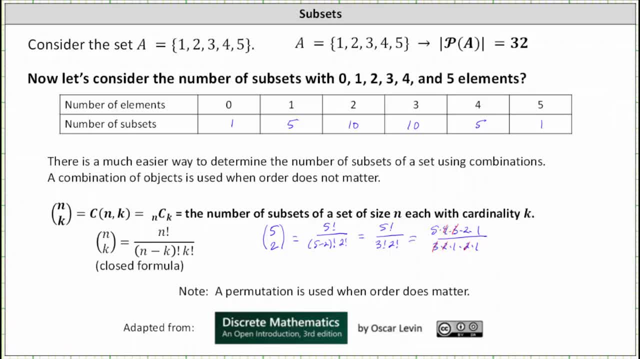 and the four in the numerator simplifies to one. Notice how this does leave us with five times two or 10, which is what we expected from the table. Set A has 10 subsets with cardinality, two or 10 subsets with two elements. 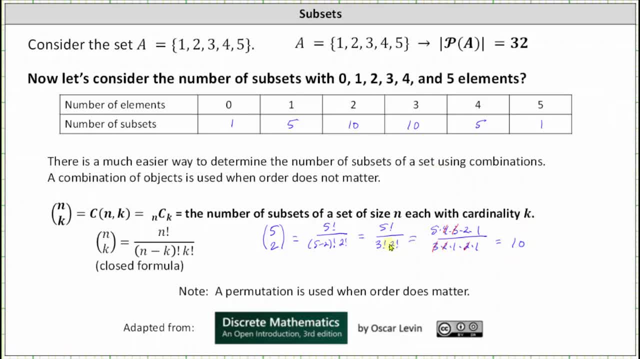 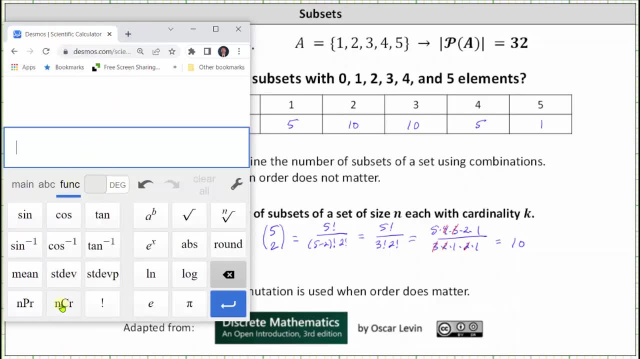 And before we go, I do want to mention most calculators do have a combination function. For example, here is the Desmos scientific calculator. If we click functions and then NCR is the combination function and then we go back to the main keyboard. 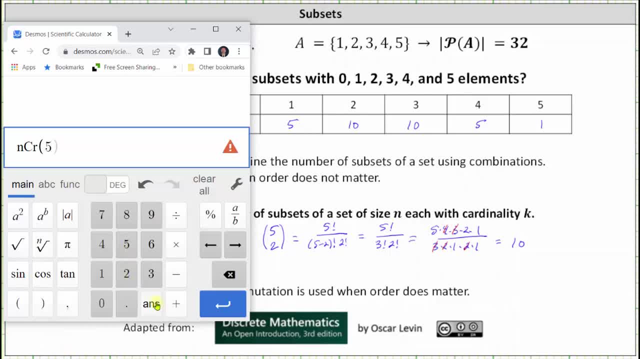 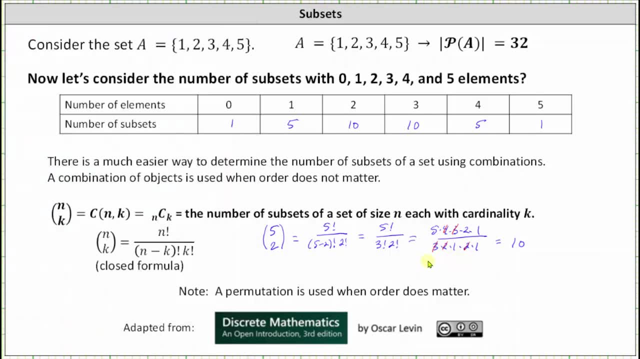 and simply enter five comma, two for five, choose two and the combination is calculated, which does verify. the result is 10.. I hope you found this helpful. 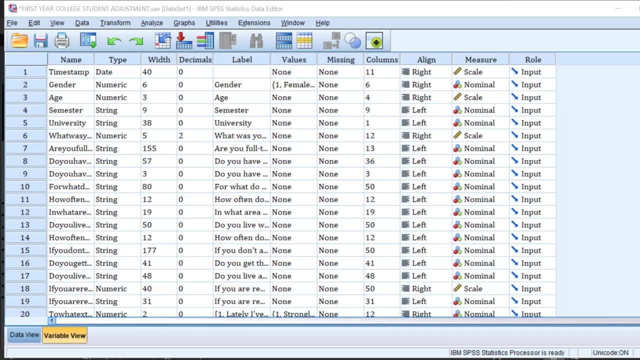 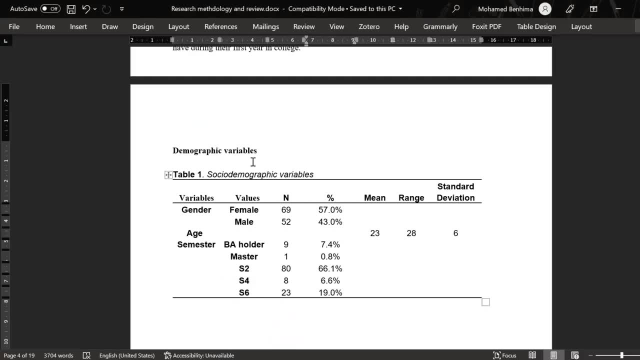 Hello, I hope you are doing great. In this tutorial I'm going to show you how you can combine demographic variables and make them into one table, like this table, which includes gender, age, semester, etc. So to do this, we can use spaces and we go to analyze and 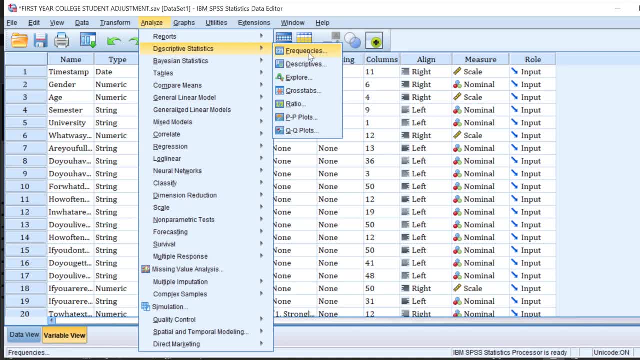 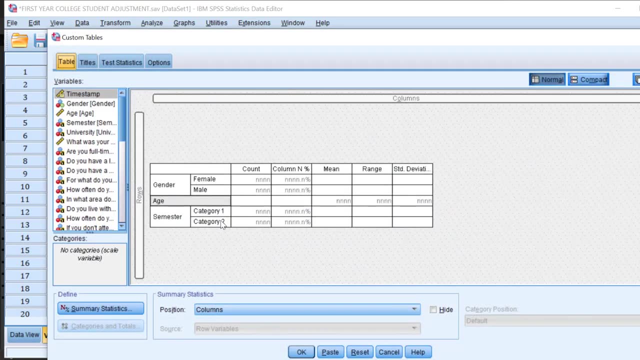 not do descriptive stats and frequencies, as most researchers do, but rather we are going to go to custom tables and then custom tables. Then I need to move these variables here so that I can put them into the row. so I will choose whether I will move them to the rows or